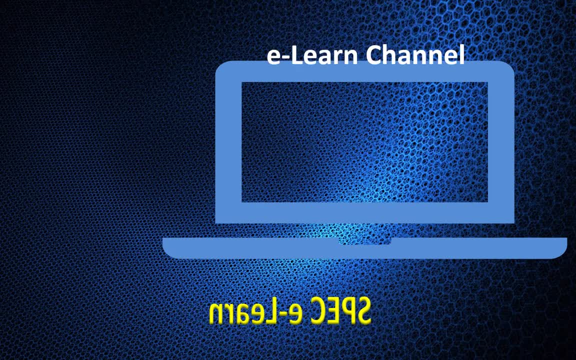 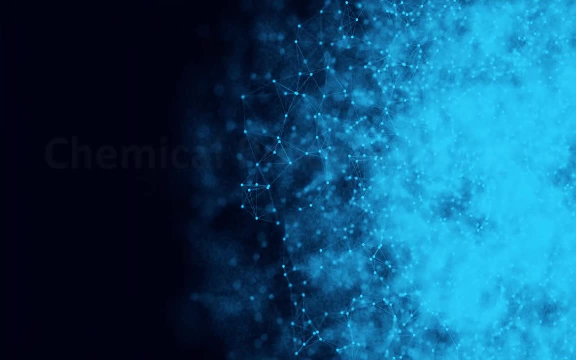 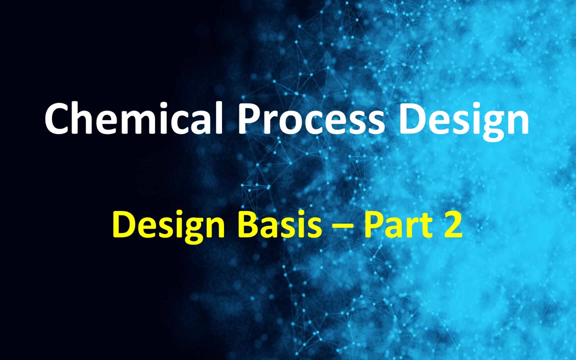 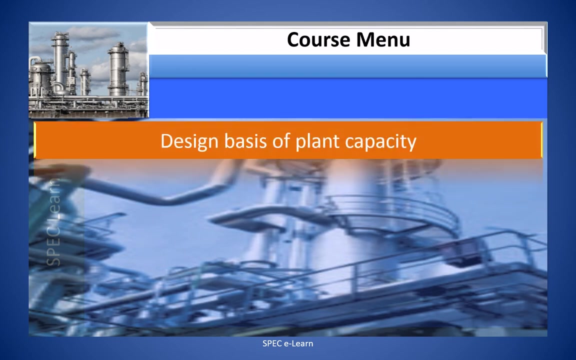 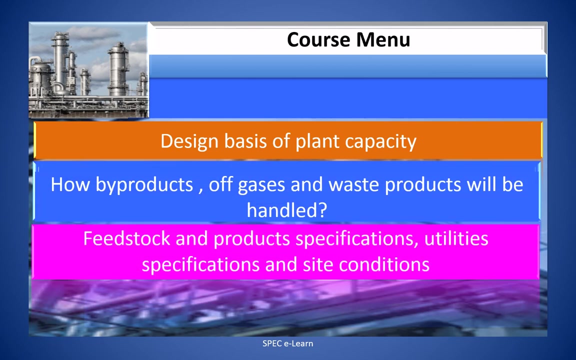 Hello everyone, welcome to SPECT eLearn, the online learning channel dedicated to chemical engineers. In this video course, you will learn the design basis of plant capacity, how by-products of gases- base products- will be handled, feedstock and product specifications, utility specifications and site conditions. 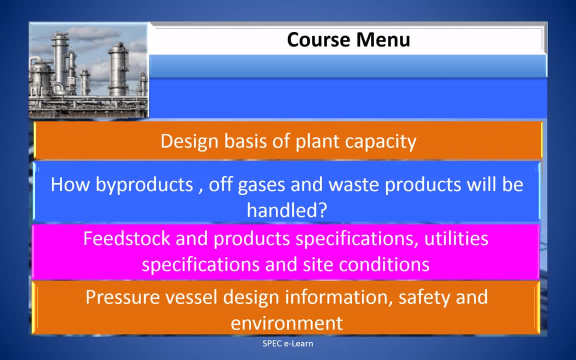 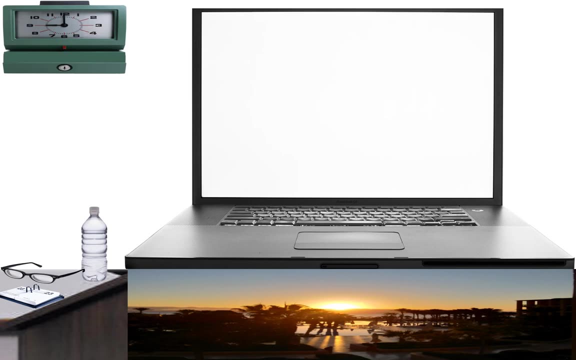 principles of design, information, safety and environment. Please subscribe to the channel. By subscribing, you will motivate us to produce knowledgeable video content for you. So subscribe now, before you forget. In the part 1 of the design basis, you understood some of the aspects of the basis of chemical process design. 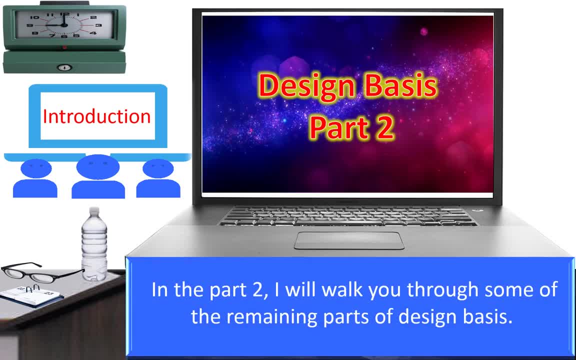 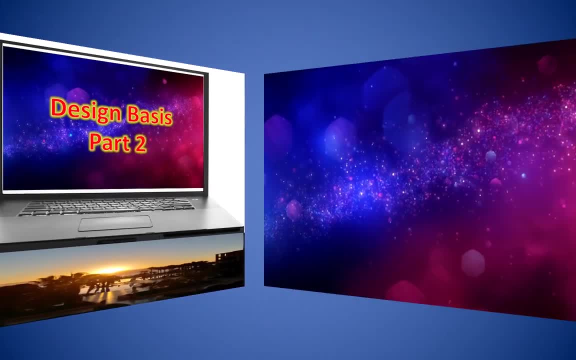 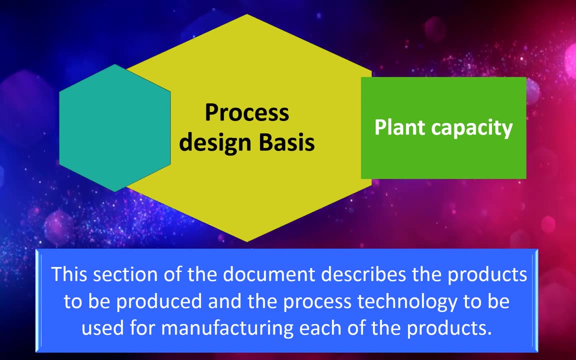 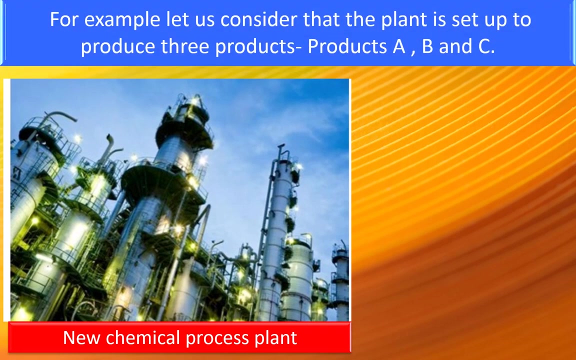 In the part 2,. I will walk you through the remaining parts of the design basis: Plant Capacity. This section of the document describes the products to be produced and the technology to be used for manufacturing each of the products. For example, let us consider that the plant is set up to produce 3 products. 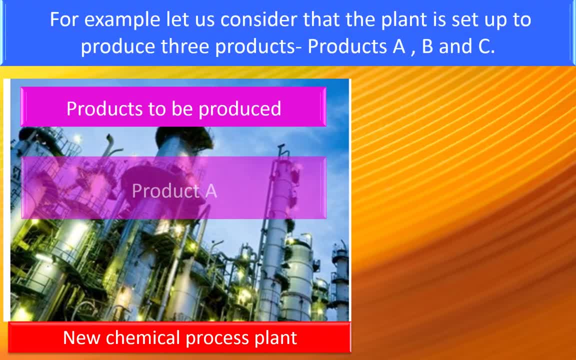 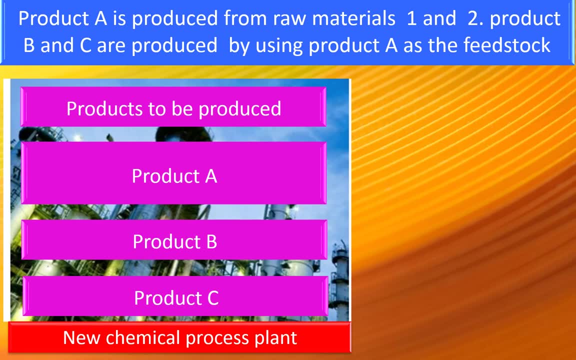 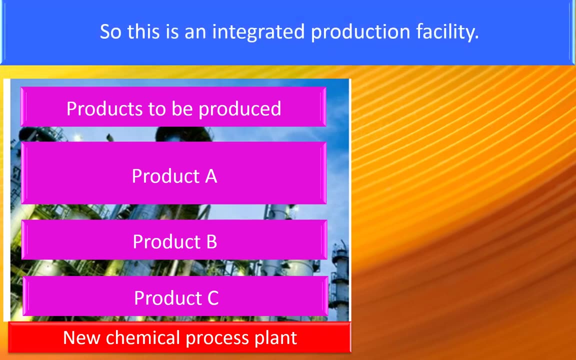 Products A, B and C. Products A is produced from raw materials 1 and 2.. Products B and C are produced by using the product A as a feedstock. So this is an integrated production facility. For each of the products, the design basis specifies the technology. 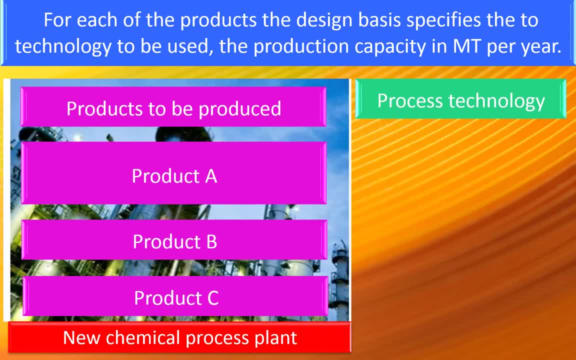 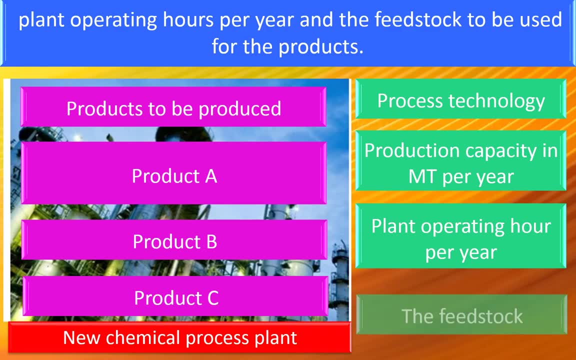 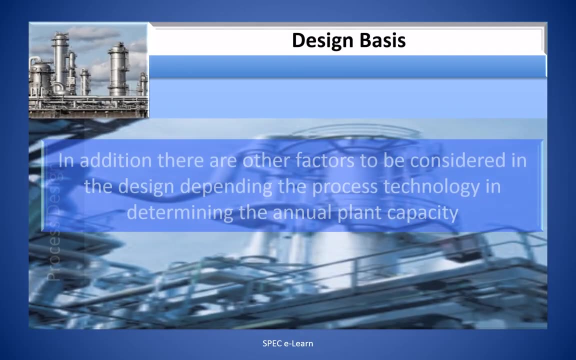 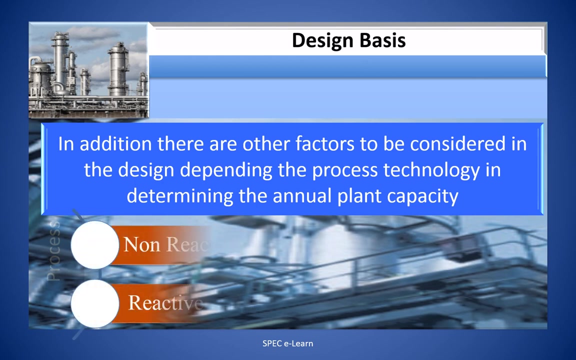 specifies the technology to be used, the processing capacity in metric ton per year, the plant operating hours per year and the feedstock to be used for the products. In addition, there are other factors to be considered in the design, depending on the process technology in determining the annual plant capacity. Non-reactive. 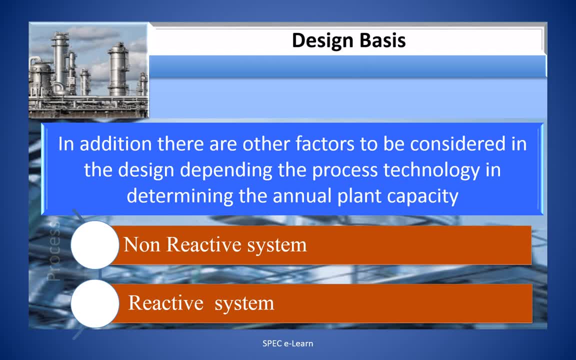 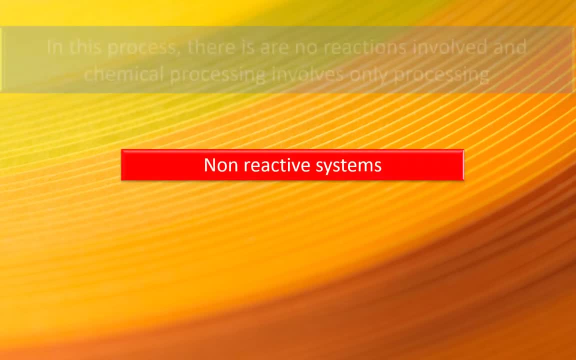 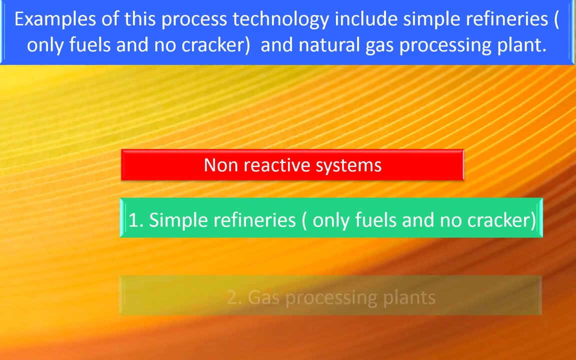 system and reactive system. Non-reactive system. In this process there are no reactions involved and chemical processing involves only processing of the feedstock using separation processes. Examples of this process technology include simple refineries, only fuels and no cracker and natural gas processing. 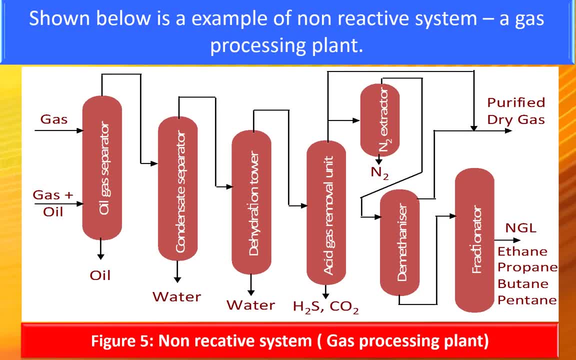 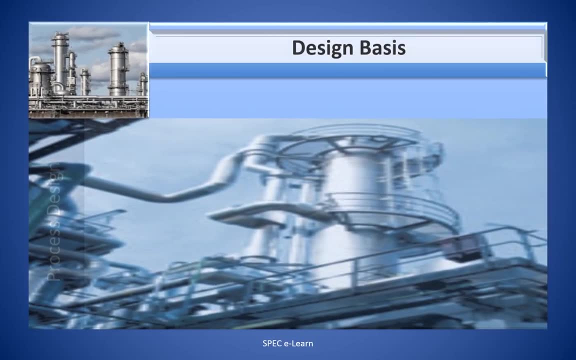 Shown below is an example of a non-reactive system: a gas processing plant. In non-reactive processes, the processing capacity for the design basis remains the same during the operating life of the plant. Reactive systems: In this process one or more feedstock undergo. 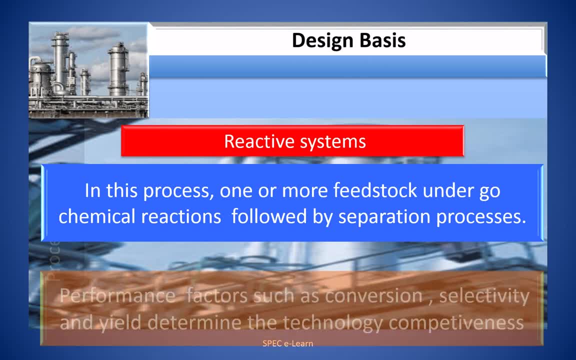 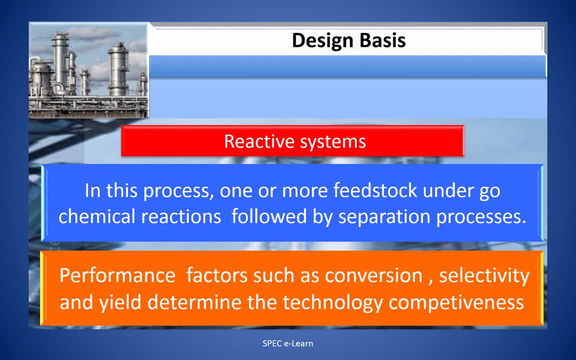 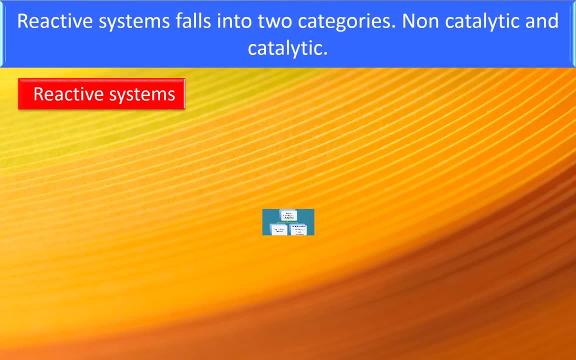 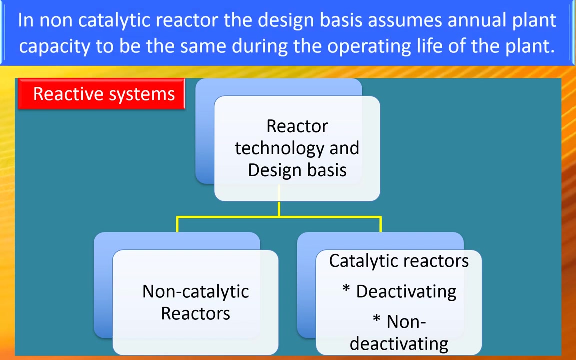 chemical reactions followed by separation processes. Performance factors such as conversion selectivity and yield determine the technology competitiveness. Reactive systems fall into two categories: non-catalytic and catalytic. In non-catalytic reactor, the design basis assumes annual plant capacity to be the same. 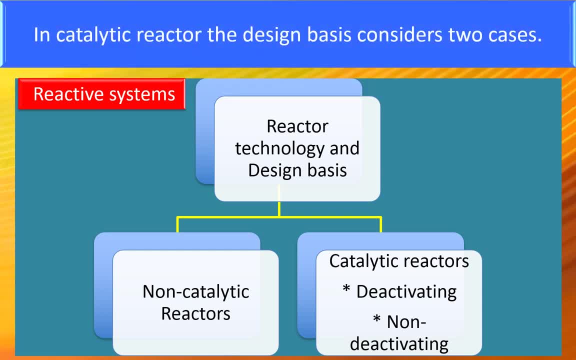 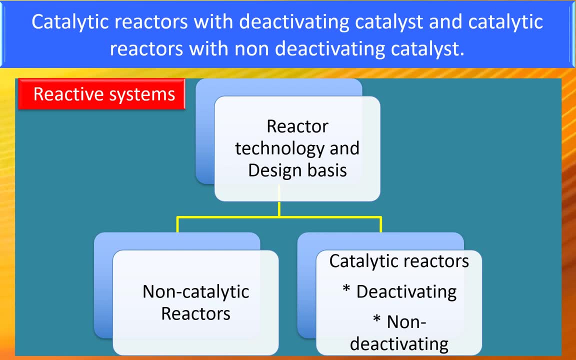 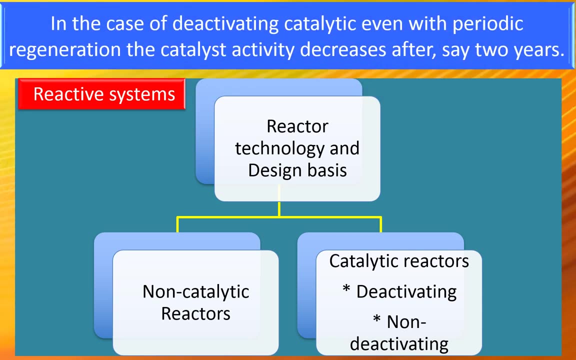 during the operating life of the plant. In catalytic reactor, the design basis considers two cases: Catalytic reactors with deactivating catalysts and catalytic reactors with non-deactivating catalysts. In the case of deactivating catalysts, even with periodic regeneration, the catalyst activity 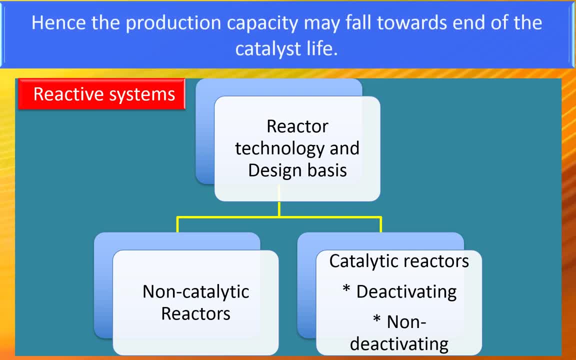 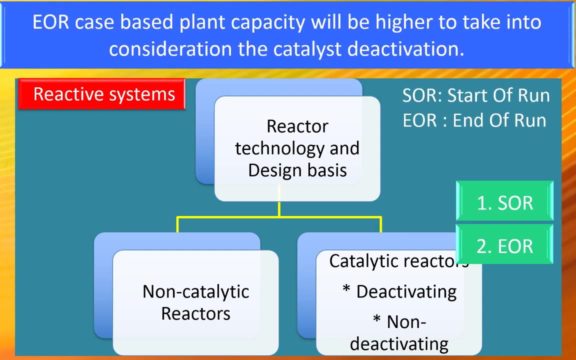 gets reduced after, say, two years. hence the processing capacity may fall towards the end of the catalyst life. This has to be considered in deciding the design basis as start of the run- SOR or end of the run- EOR. EOR: case based plant capacity will be higher to take into consideration the catalyst deactivation. 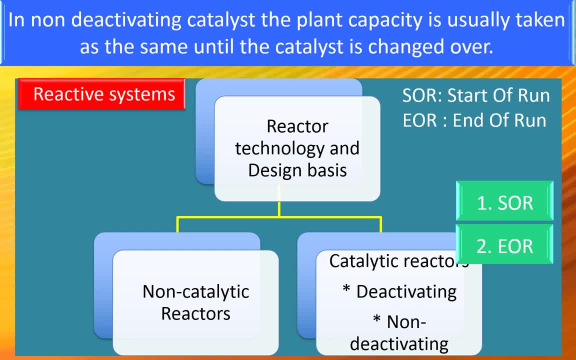 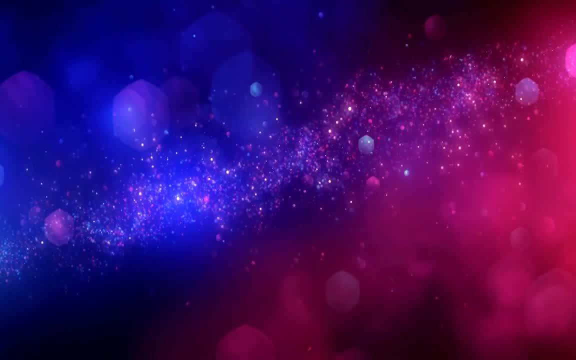 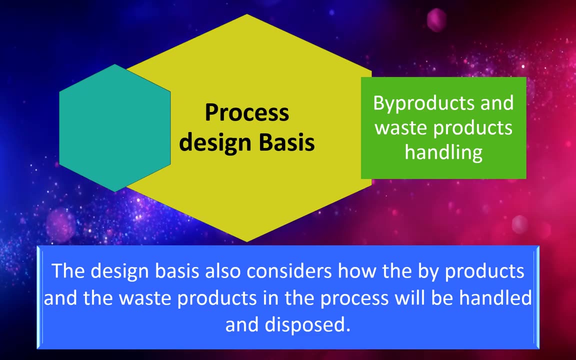 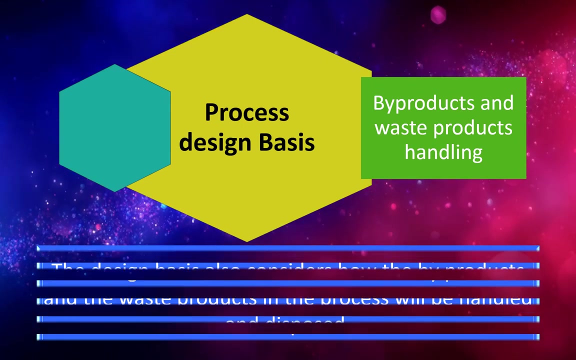 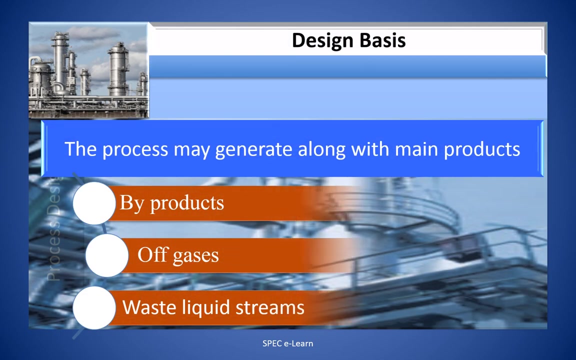 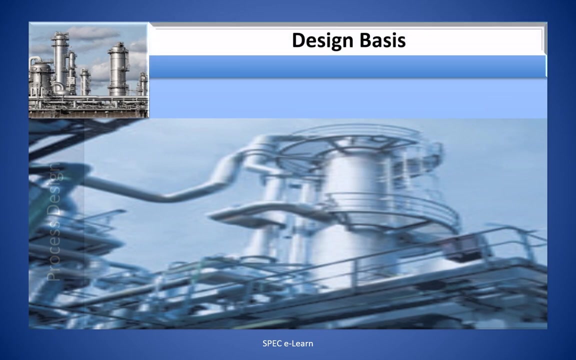 In non-deactivating catalyst, the plant capacity is usually taken as the same until the catalyst is changed over. Byproducts and waste products handling. The design basis also considers how the byproducts and the waste products in the process will be handled. The process may generate, along with main products, byproducts, off-gases and waste liquid streams. 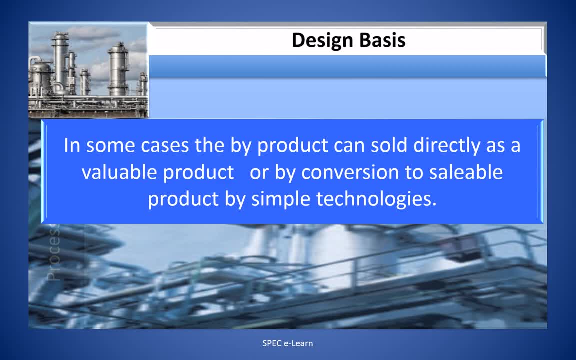 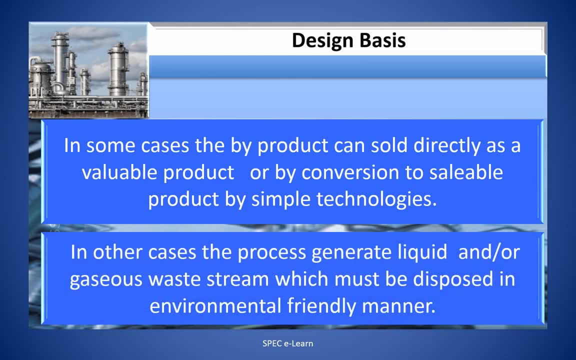 In some cases, the byproduct can be sold directly as a valuable product or by conversion to saleable product by simple technologies. In other cases, process generate liquid and or gaseous waste streams, which must be disposed in environmentally friendly manner. This will be clearly specified with the. 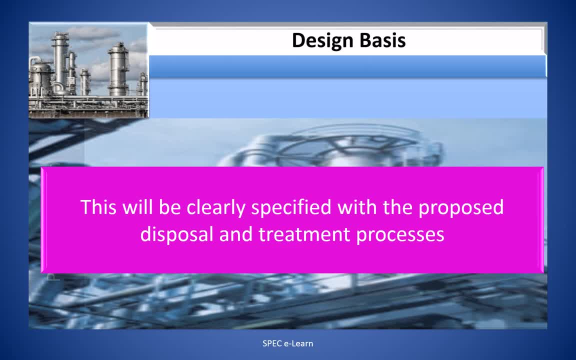 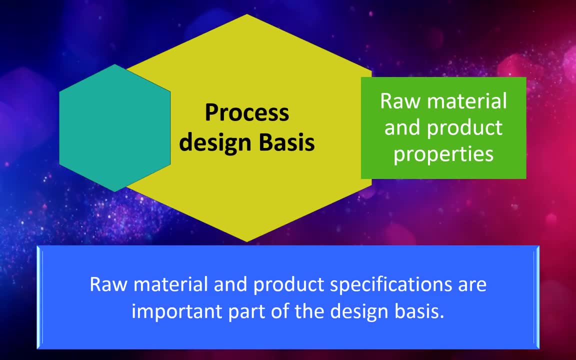 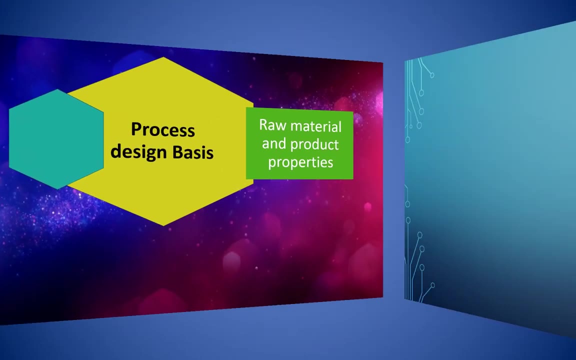 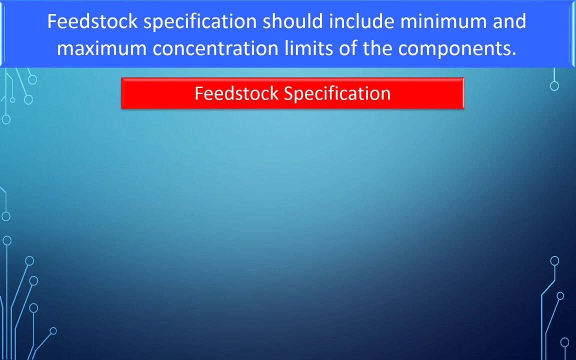 proposed disposal and treatment processes. Raw material and product properties. Raw material and product specifications are important part of the design basis. Feedstock specifications should include minimum and maximum concentration limits of the components. The minimum concentration of the principle reactant should be specified. 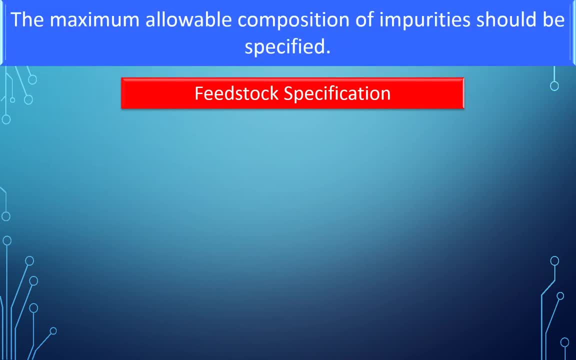 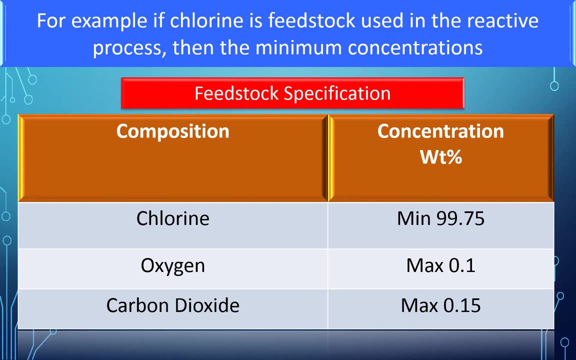 The maximum allowable composition of impurities should be specified. For example, if chlorine is a feedstock used in the process, then the minimum concentration of chlorine should be 99.75% and maximum concentration of the impurities should not be more than 0.1% oxygen and 0.15% CO2.. The physical 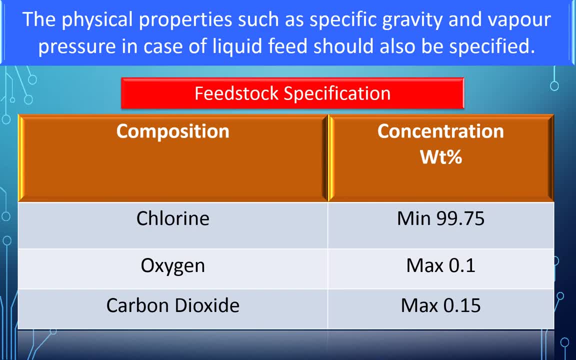 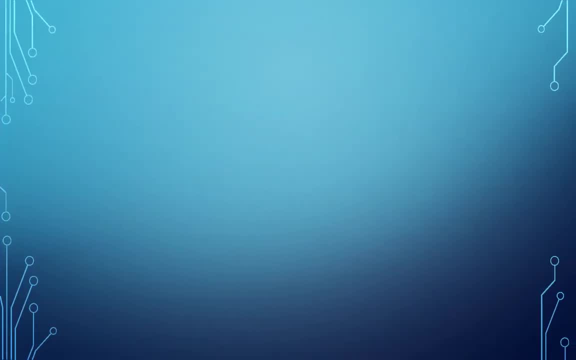 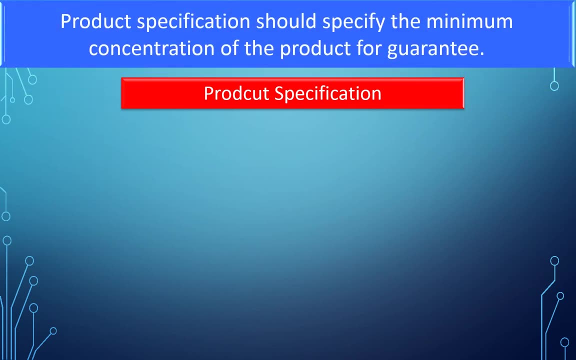 properties such as specific gravity and vapor pressure in the case of liquid feed should also be specified. Product specification: The product specification should specify the minimum concentration of the product. for guarantee. Maximum concentration of impurities should be specified, including water content, For example, if the product is allyl chloride. the specification 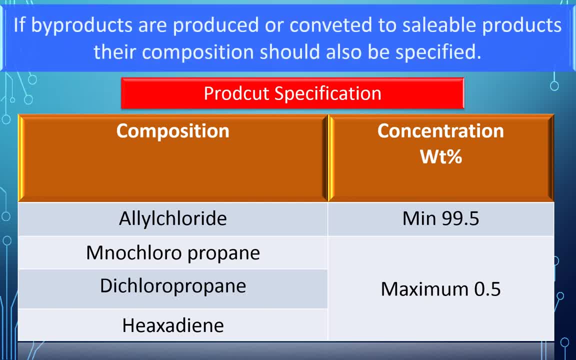 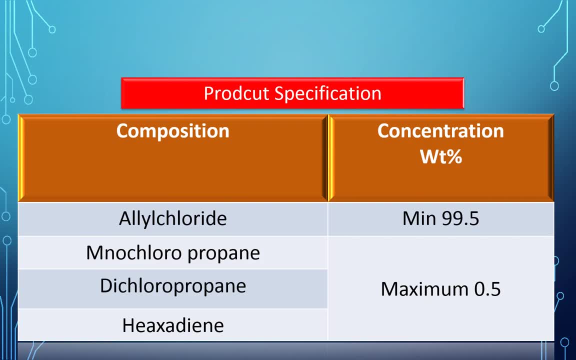 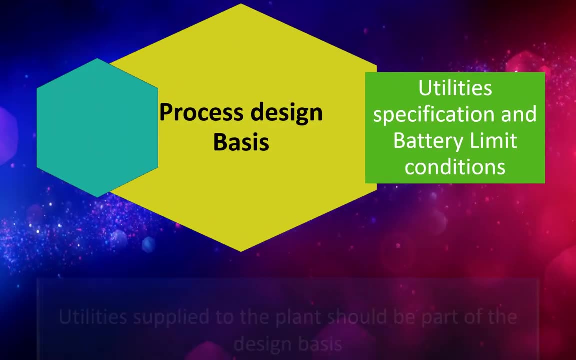 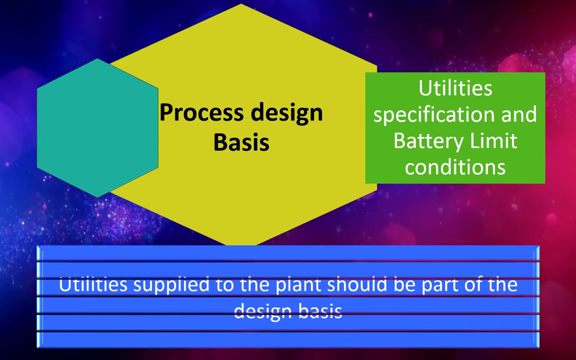 will be as shown in the table below. If by-products are produced or converted to saleable products, their composition should also be specified. Utility specification And battery limit conditions: Utilities supplied to the plant should be part of the design basis. Before we move on, I would like to make a call to my dear viewers. 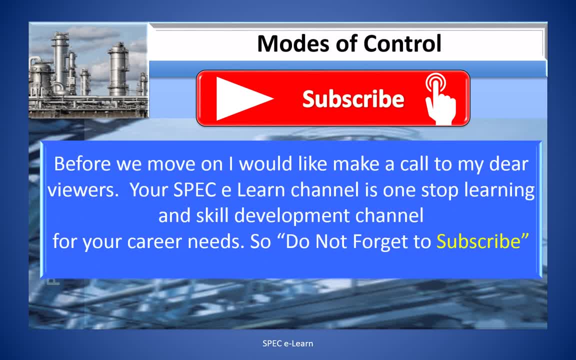 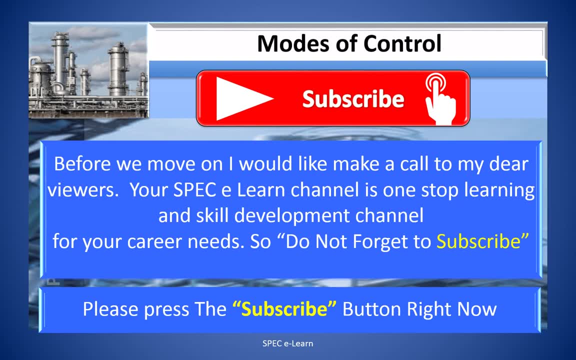 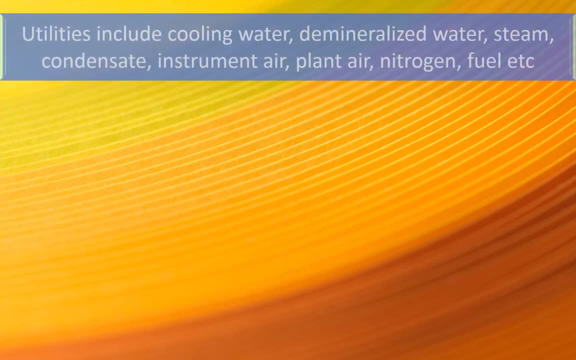 Your SPEC eLearn channel is a one-stop learning and skill development channel for your career, So do not forget to subscribe. Please press the subscribe button right now. Utilities include cooling water, demeralized water, steam, condensate instrument, air plant air. 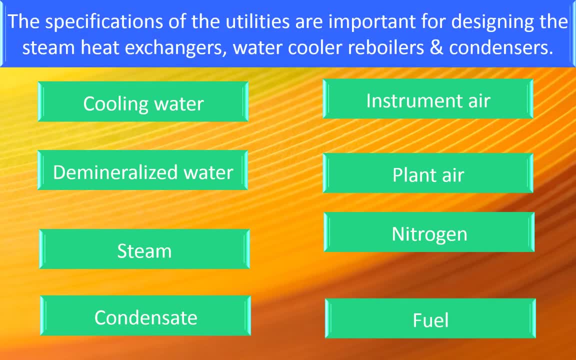 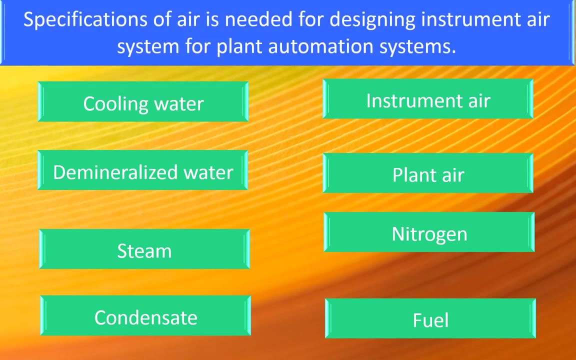 nitrogen fuel, etc. The specification of the utilities are important for design of the steam heat exchangers, water coolers, reboilers and condensers. Specification of air is needed for designing instrument air system for plant automation system. 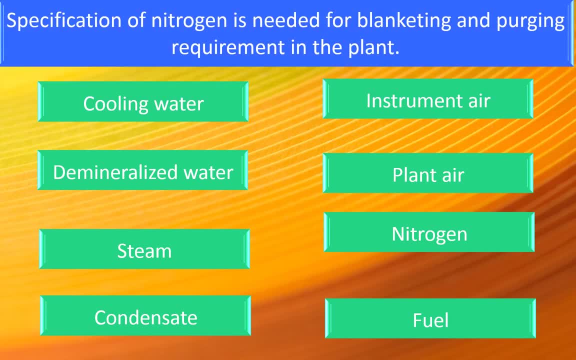 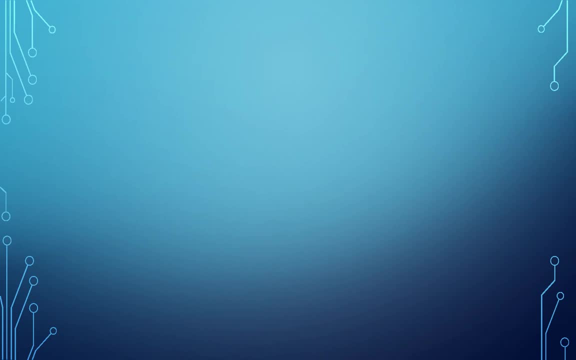 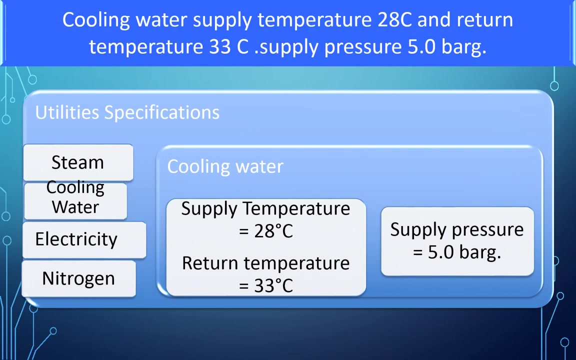 Specification of the system of the plant can be used to design of the plant automation systems. Nitrogen is needed for blanketing and purging requirement in the plant. Typical specifications of utilities for design basis is as shown in the table below: Cooling water supply temperature 20 degree centigrade and return temperature 33 degree. 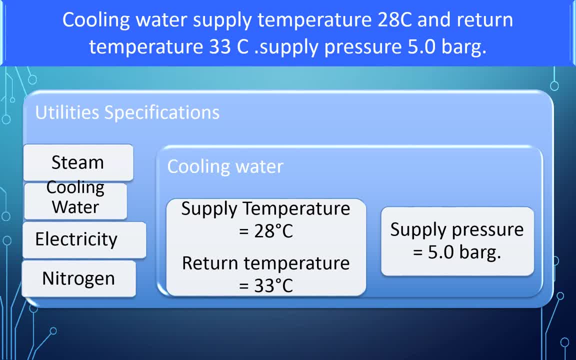 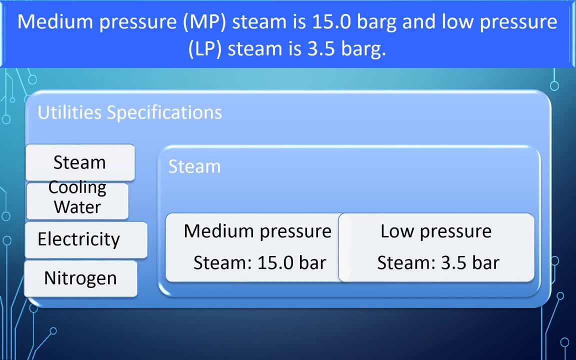 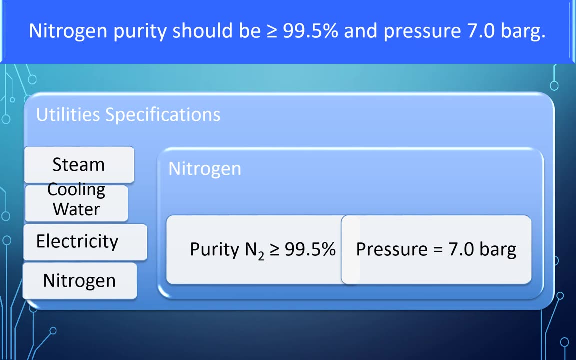 centigrade and supply pressure 5 bar g. Medium pressure stream is 15 bar g and low pressure stream 3.5 bar g. Nitrogen purity should be greater than or equal to 99.5 percent and pressure 7 bar g. Specification for electricity is high voltage, 3.3 kV. 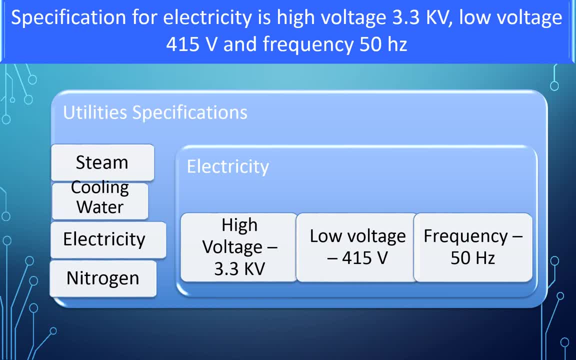 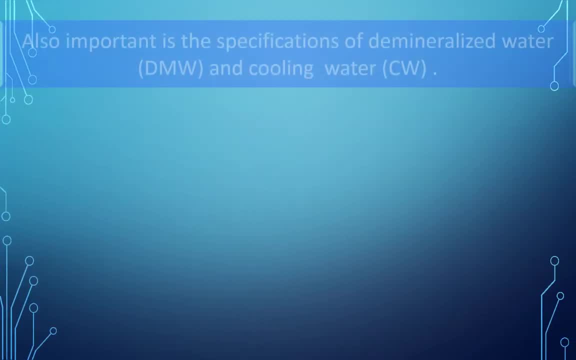 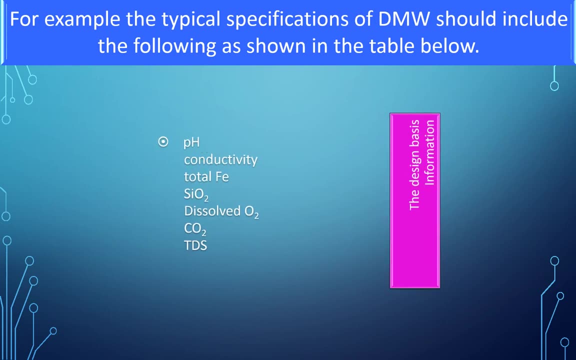 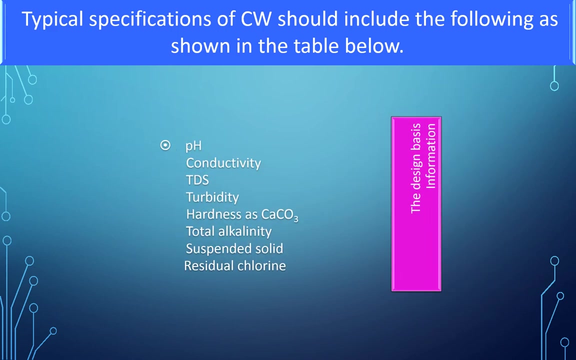 low voltage 415 volts and frequency 50 hertz. Also important is a specification of demonetized water and cooling water. For example, the typical specification of DM water should include the following, as shown in the table below. Typical specifications of cooling water should include the following, as shown in the table below. 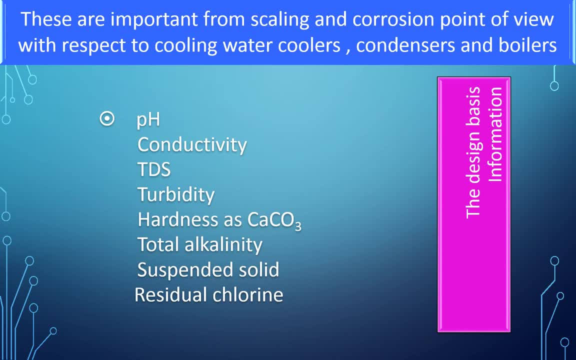 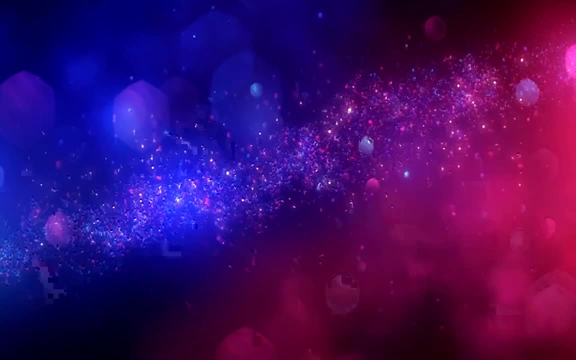 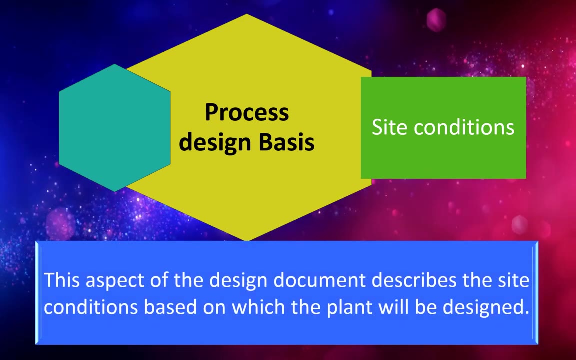 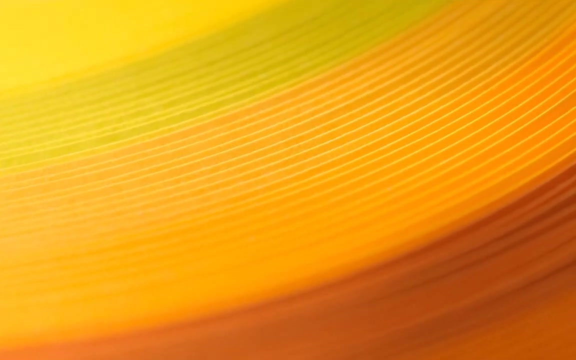 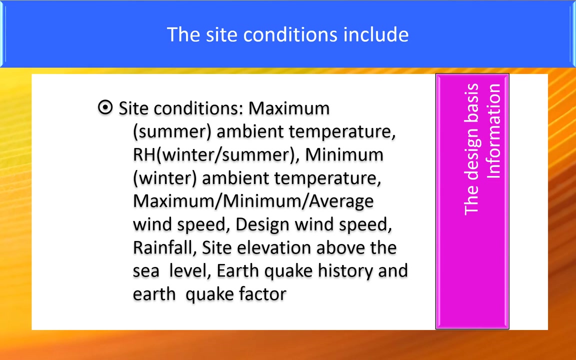 These are important from scaling and corrosion point of view with respect to cooling water coolers, condensers and boilers. Site conditions: This aspect of the design document describes the site conditions based on which the plant will be designed. Site conditions include maximum or summer ambient temperature, relative humidity, winter and summer. 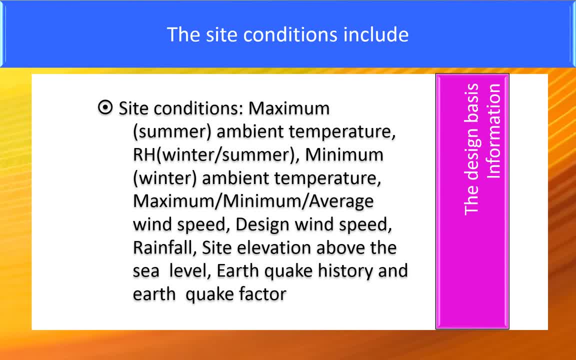 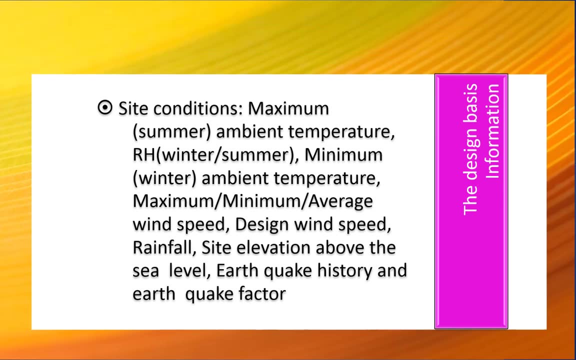 minimum or winter ambient temperature. maximum, minimum and average wind speed design wind speed, rainfall, site elevation, temperature and temperature. The site conditions are the following: Site elevation above the sea level, earthquake history and earthquake factor. Pressure vessel design information. 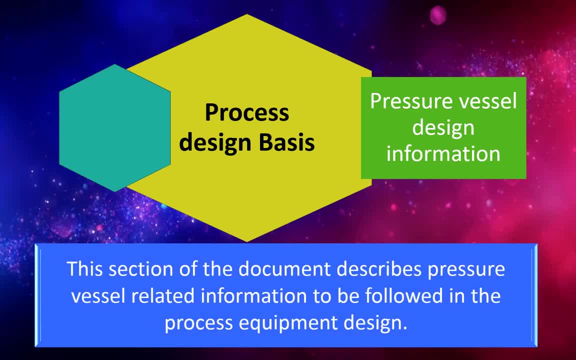 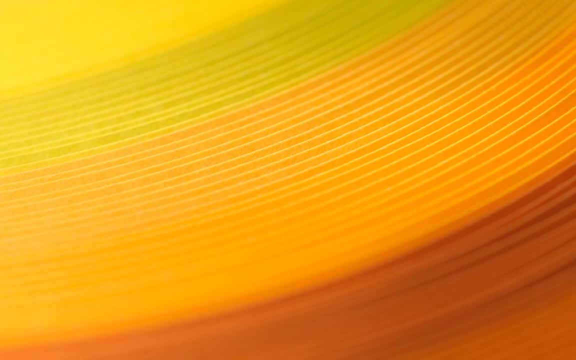 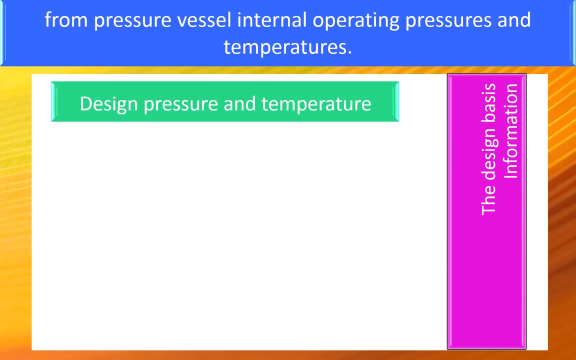 This section of the document describes pressure vessel related information to be followed in the process equipment design. The design basis document will describe how the design, pressure and temperature will be determined From the pressure vessel internal operating pressures and temperatures. Material of construction will be specified depending on the tariff conditions. 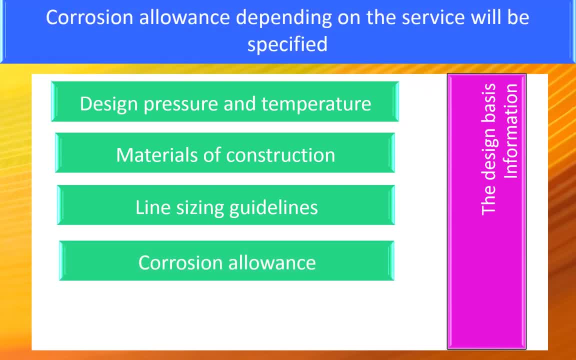 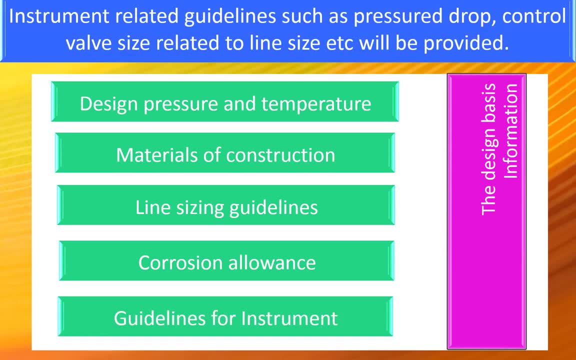 Line sizing criteria is specified. Corrosion allowance, depending on the service, will be specified. Instrument related guidelines, such as pressure drop, the control valve size, whatever ARIN ON 条, closures diameter of음. Use them in construction Vessels and tanks. 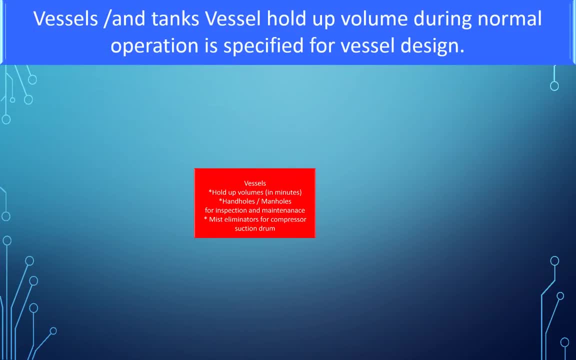 content of each type of vessel and tank system shall be included with this system audit. the message given by �on system maiden investment or to major links to further conversion with톡 request from you. Vessel hold up volume during normal operation is specified for vessel design. 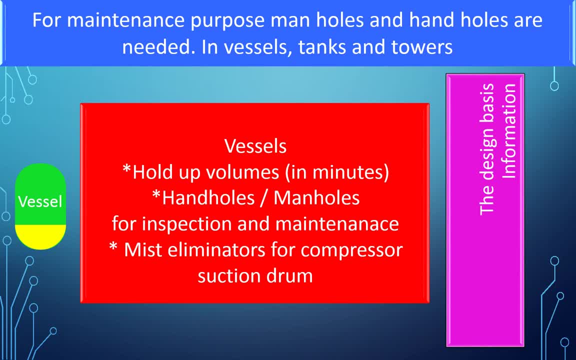 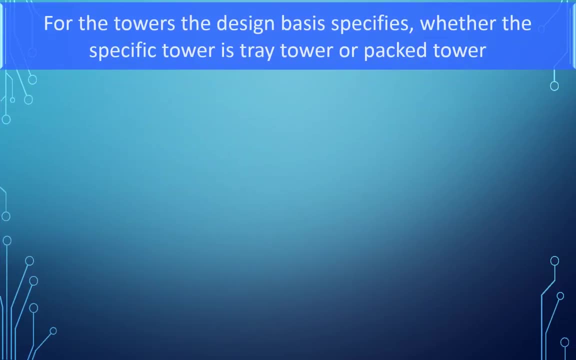 For maintenance purpose. manholes and handholds are needed in vessels and tanks and towers. They are specified for individual equipment depending on the size of the vessel or tower. For the towers, the design basis specifies whether the specific tower is a tray tower or a pack tower. 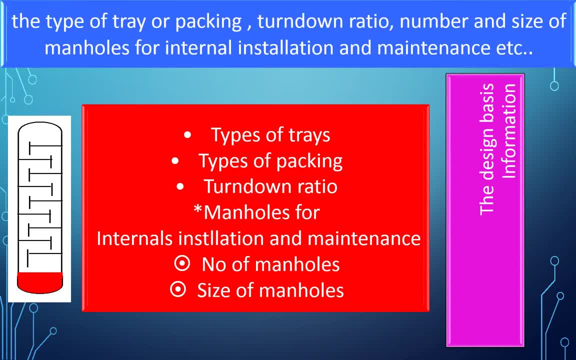 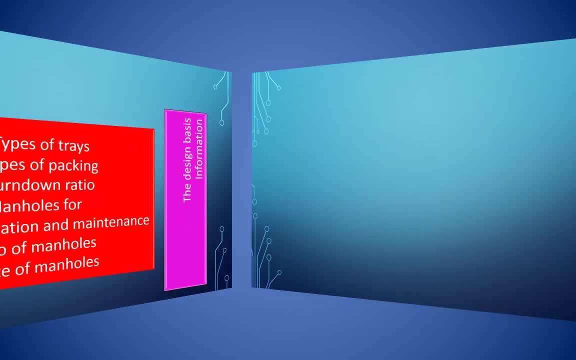 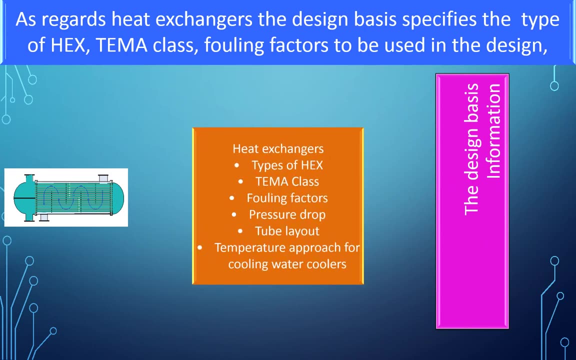 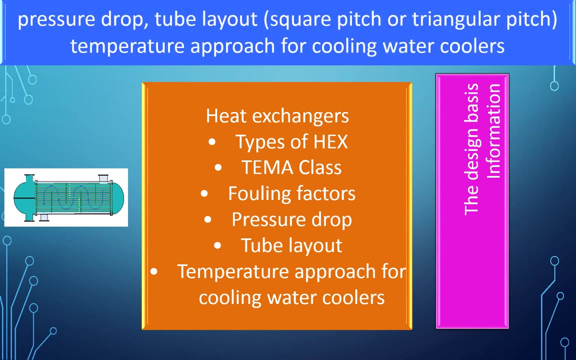 The type of tray or packing, the turn down ratio, number and size of the manholes for internal installation and maintenance, etc. As regards heat exchangers, the design basis specifies the type of heat exchanger- T-mark cloths, fouling factors to be used in the design. pressure drop tube layout square. 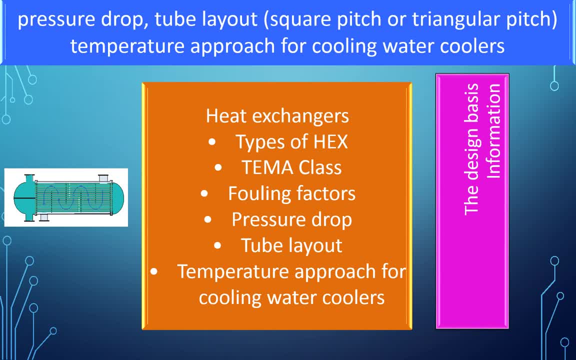 pitch or triangular pitch. temperature approach for cooling water coolers. The design basis specifies the type of heat exchanger- T-mark cloths, fouling factors to be used in the design. pressure drop tube layout- square pitch or triangular pitch. 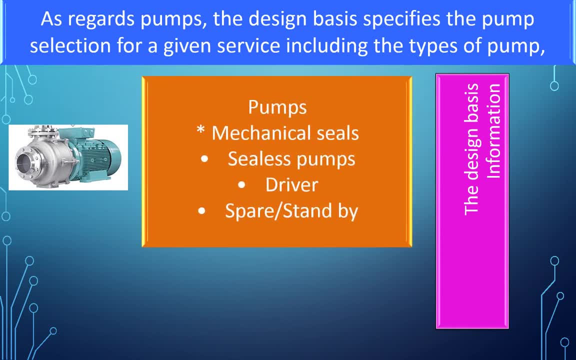 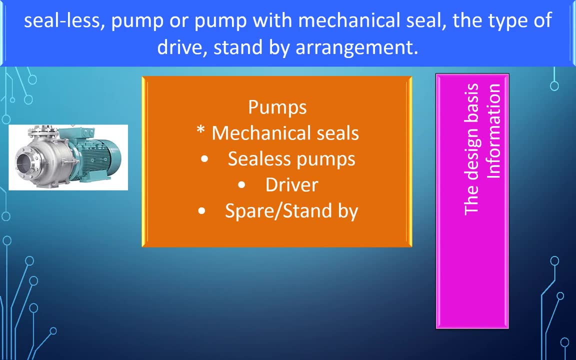 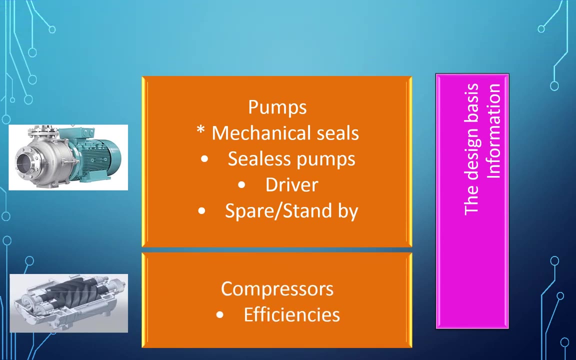 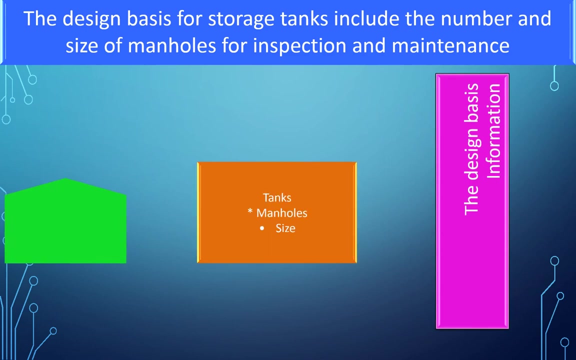 As regards pumps, the design basis specifies the pump selection for a given service, including the type of pump- realise pump or pump with mechanical seal- the type of drive, standby arrangements, etc. For compressors, the efficiencies are specified. The design basis for the storage tanks include the number and size of manholes for inspection. 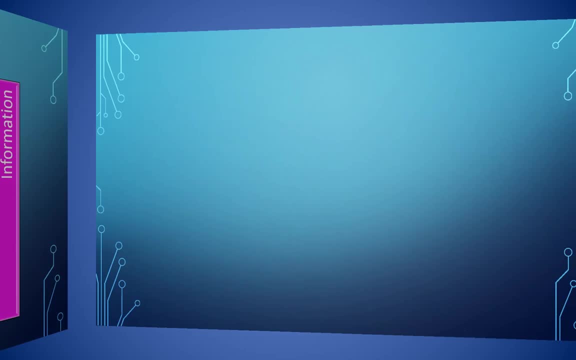 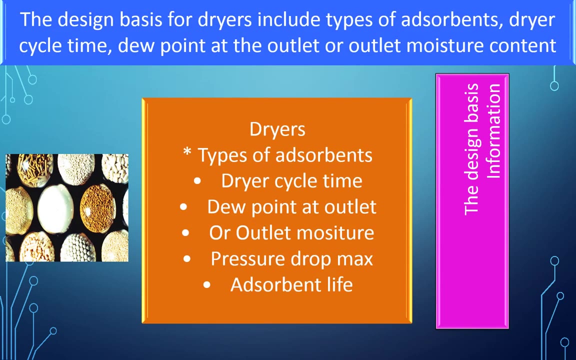 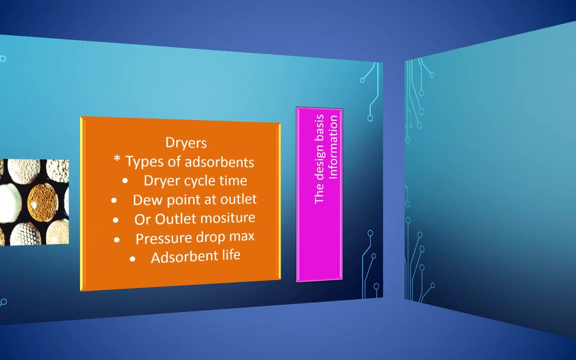 production and maintenance. Dryers or dehydration tubbers are used in the separation processes. The design basis for the dryers include types of adsorbents, dry cycle time, dew point at the outlet or outlet, moisture content, maximum pressure drop allowable and adsorbent life. 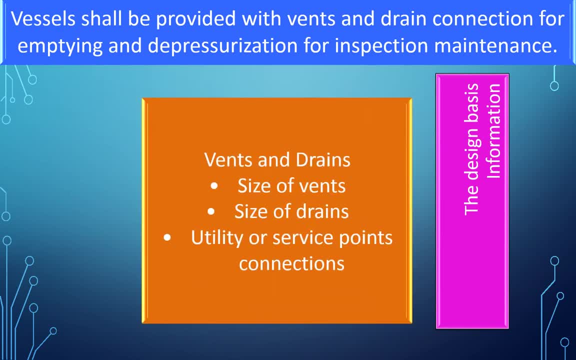 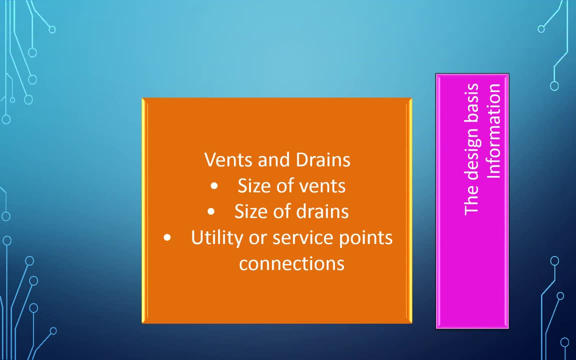 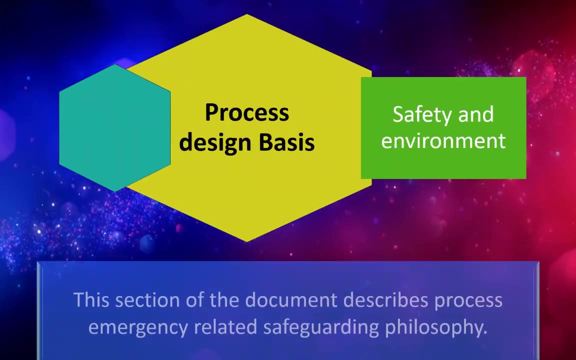 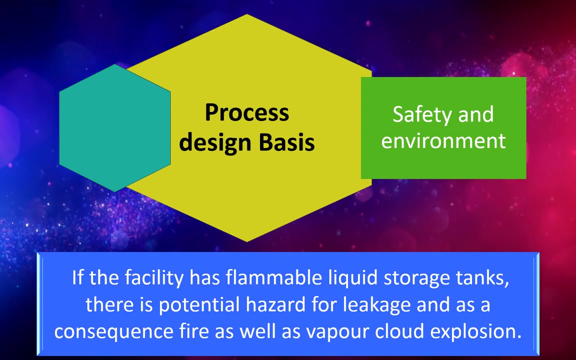 Sales shall be provided with vanes and drain connections for emptying and deprecation for inspection and maintenance. Also specifies a connection for utility services, Safety and environment. This section of the document describes the process emergency related safeguarding philosophy. If the facility has flammable liquid storage tanks, there is a potential hazard for leakage. 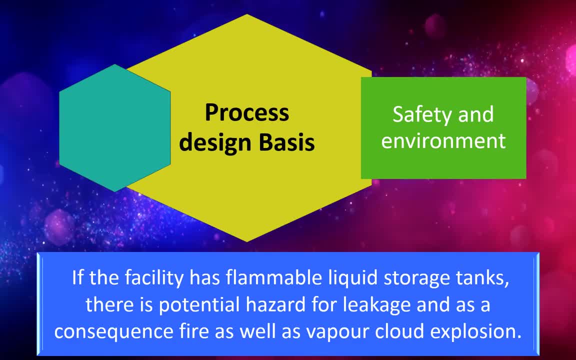 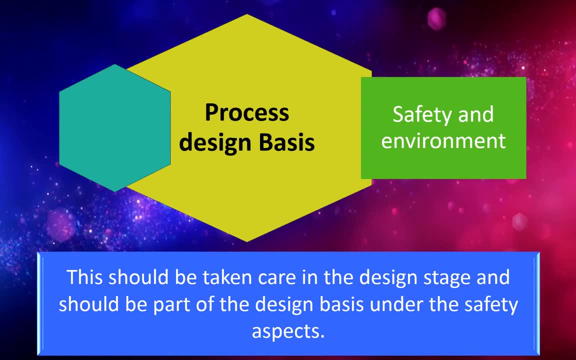 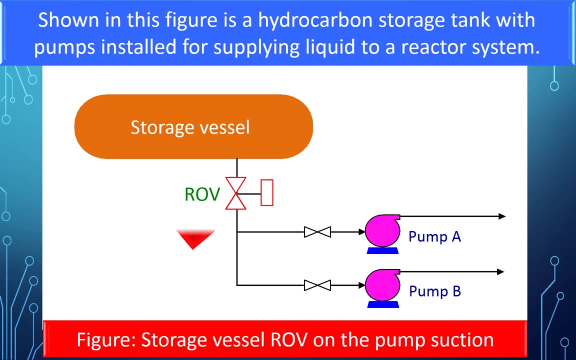 and, as a consequence, fire as well as vapor cloud explosions. This should be taken care in the design stage and should be part of the design basis under safety aspects. Shown in this figure is a hydrocarbon storage tank with pumps installed for supplying liquid to a reactor system.